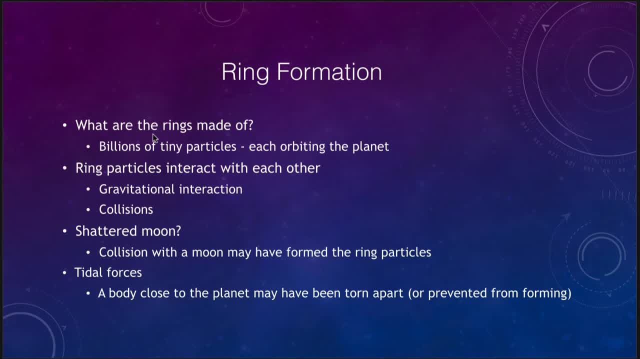 Where do rings come from in the first place? Well, first of all, what are the rings made up of? They are billions of tiny particles each orbiting the planet. You can think of them each as a small moon. So there's a small moon orbiting each planet. 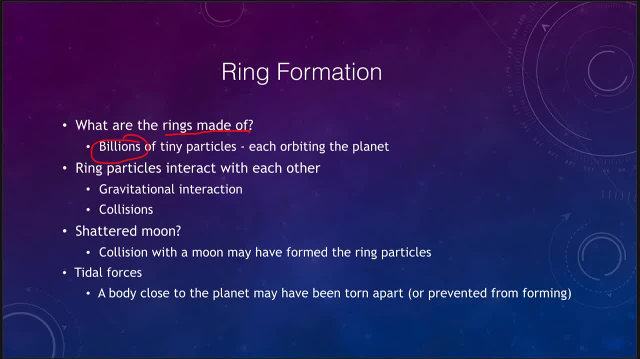 and each of these is very small objects. They may only be a few centimeters in size. They may be up to a meter or so in size, but they're not gigantic objects by any sense. The ring particles do interact with each other by gravity, which keeps them together. 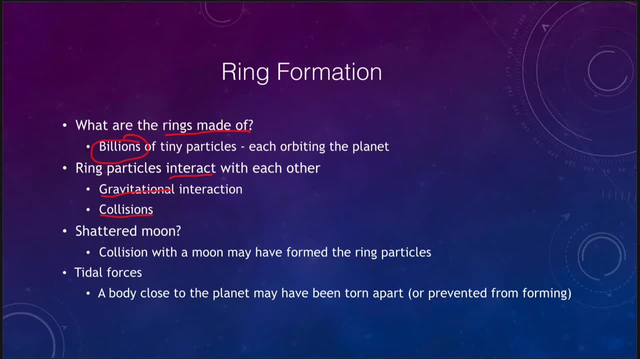 and through collisions. So the particles will collide together as they orbit and that will give us the structures that we will see within the rings. Could these be a shattered moon? A collision with the moon might have formed the ring particles. So if a large object crashed into a moon, 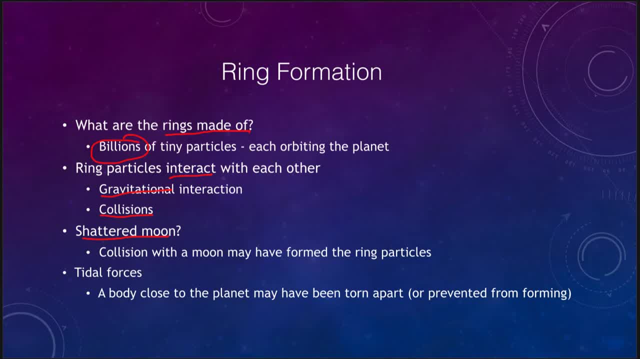 and recall that these Jovian planets all have lots of moons that could have expelled a lot of ring particles out into space that could have been captured in a ring, So perhaps some sort of collision with the moon or tidal forces as well. 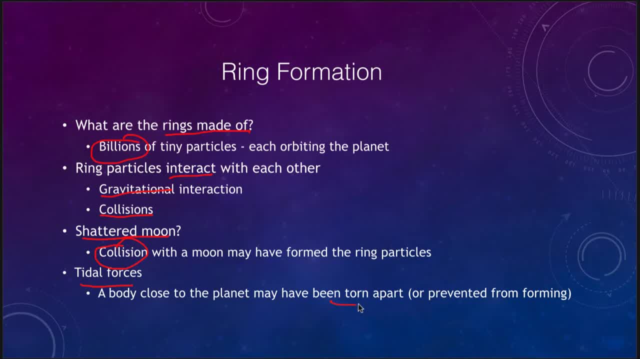 An object that gets close enough to the planet could have been torn apart by its tidal forces, The gravity on one side of the object, the near side, being stronger than the gravity on the far side, because the gravitational force depends on distance. If you're close enough to the object, 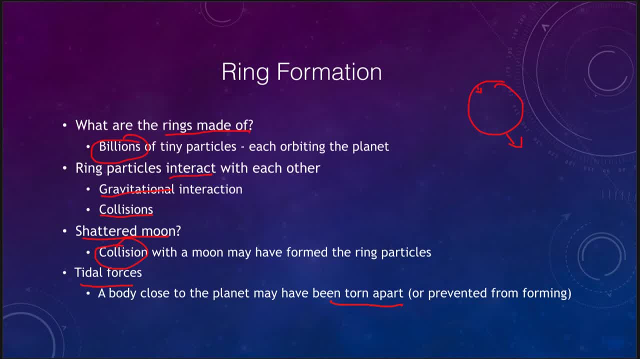 it's quite possible that the object will not be able to hold up structurally to a significant force on one side and a very small force on the other. Essentially, you're strapped, You're stretching the object apart And in case if particles are just that close? 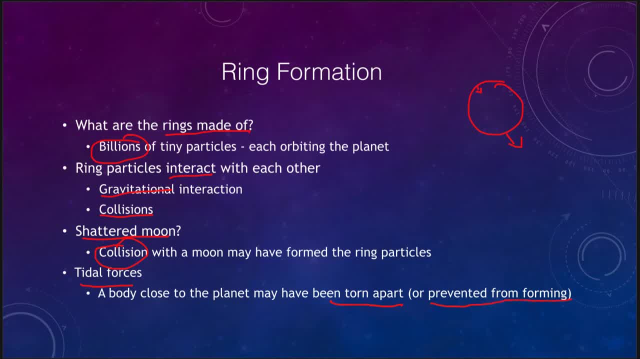 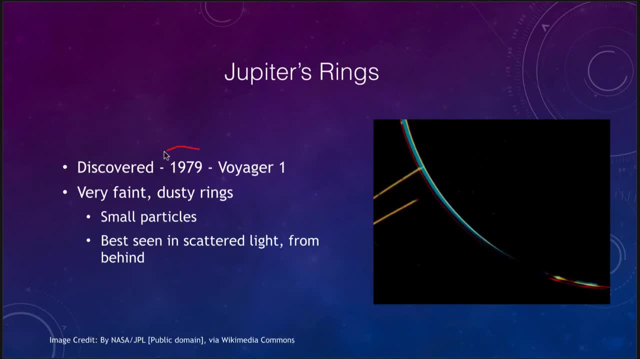 it may just have been prevented from forming in the first place. So let's look at the rings of each of these planets. So starting off here with Jupiter's rings, which were discovered in 1979 by the Voyager 1 spacecraft. They are very faint and dusty rings. 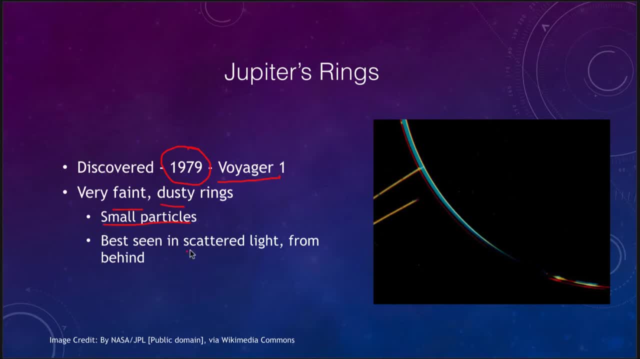 made up of lots of small particles and are best seen in scattered light from behind. So we don't see them. We don't see them at all from Earth because they're not reflecting a lot of the light, but they do scatter the light through. 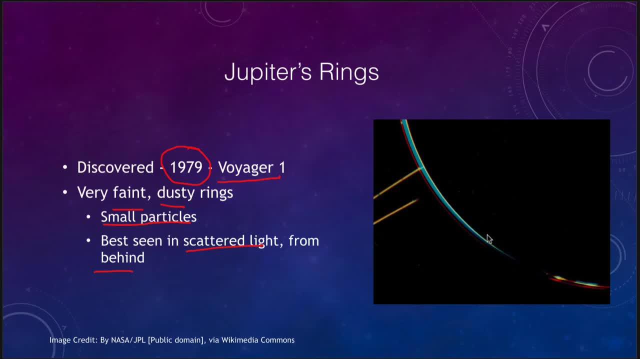 And if we look from behind Jupiter, as seen by the Voyager 1 craft, we can see the dark, unilluminated side of Jupiter here. And then we're looking through towards the sun and we can see the very thin illuminated ring part. 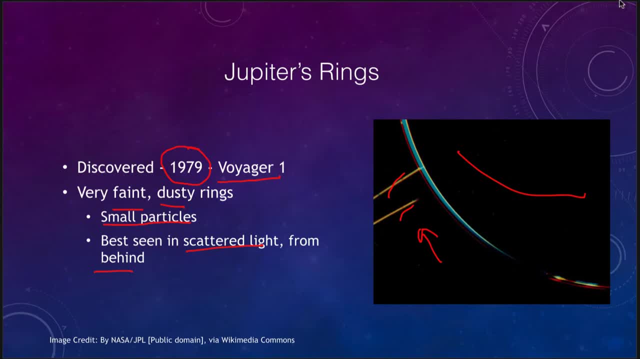 right here going around Jupiter. So Jupiter does have this very faint ring, but not a lot of detail there. So what we really want to look at are the rings of Saturn. Rings of Saturn have a lot more detail to them And we can see some of that here. 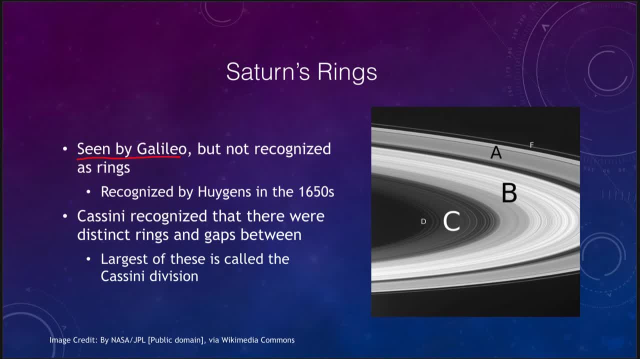 They were actually seen by Galileo, but not recognized as rings, only as a blob on each side of the planet that sometimes disappeared By the time telescopes got a little bit bigger. just a few decades later, in the 1650s, Huygens was able to recognize them as a ring system. And around that time it was a little bit bigger. It was a little bit bigger, And around that time it was a little bit bigger And around that time it was a little bit bigger. that time or a little bit later. 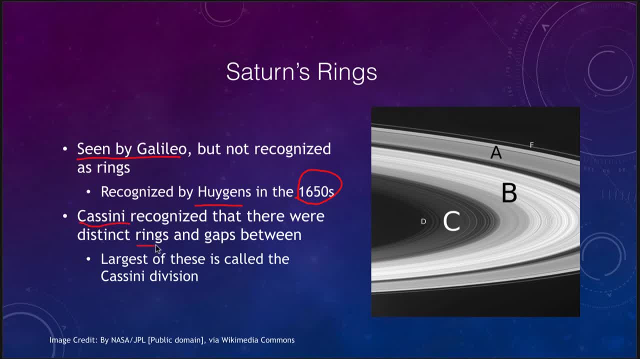 Cassini recognized that there were distinct rings, not just a single ring, and gaps between them, So gaps in between the rings. the largest of these is now named the Cassini division in his honor. So here we see the A, B, C, D and F rings out here: 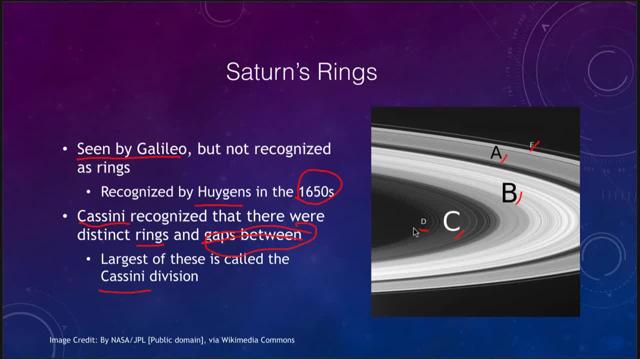 Primary ones visible that you'll see are the A, B and C. D ring is a lot fainter and harder to see. F ring is a very thin ring out beyond the A ring and also a little bit harder to see. So when we look at the structures of these rings, 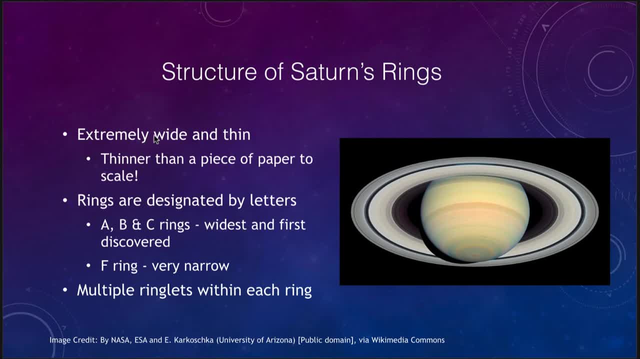 we see that they are extremely wide and thin. In fact, they are thinner than a piece of paper if you took them to scale. So if you scaled them down to a size of paper, they would be incredibly thin, much, much thinner than that piece of paper. 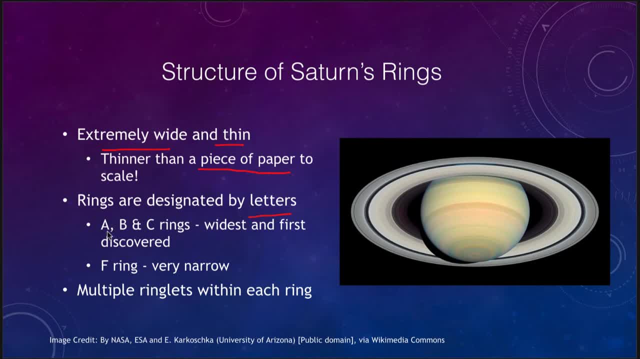 We designate the rings by letters. They are the primary ones, or the A, B and C rings, the first three to be discovered, And those are the primary widest rings that we see And those are the big bright ones there. And you also have the Cassini division, the gap. 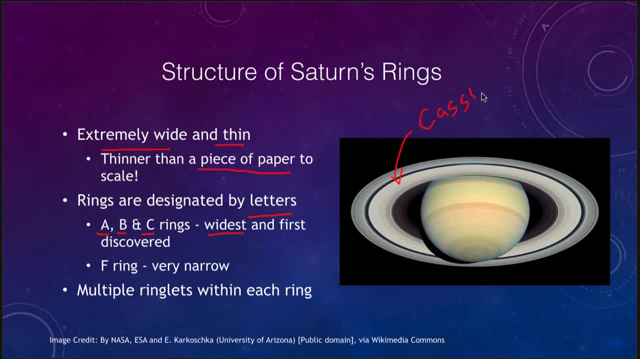 in between those rings too. So there are gaps, and not just the Cassini division, but you can see that there's another one out here, And there are other gaps and structures within the rings as well. So the rings are not just a single ring. 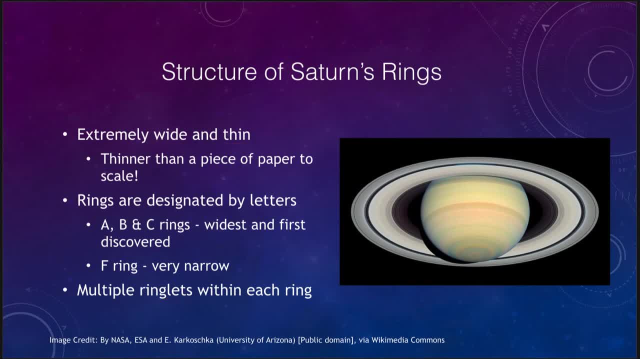 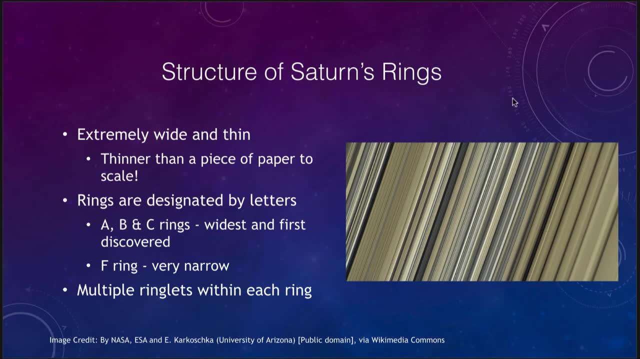 but actually have multiple ringlets within each ring. And if we look a little bit closer here, zoom in on the rings, essentially we can see that there are all kinds of structures here, little gaps and areas where there are a lot more particles. 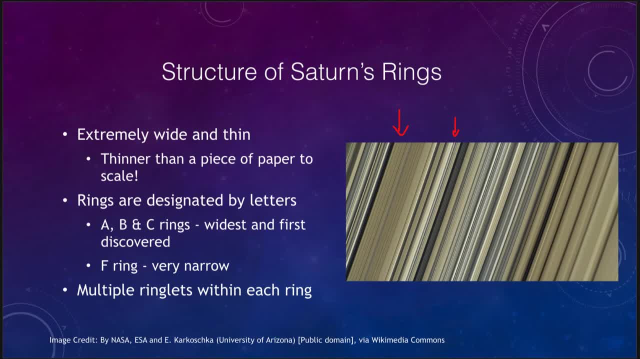 brighter areas. So big detail towards what the rings are. There's a lot of structures there And when you think about it, within each of these are just billions of particles all orbiting around Saturn and kept there. So why do they have this detailed structure? 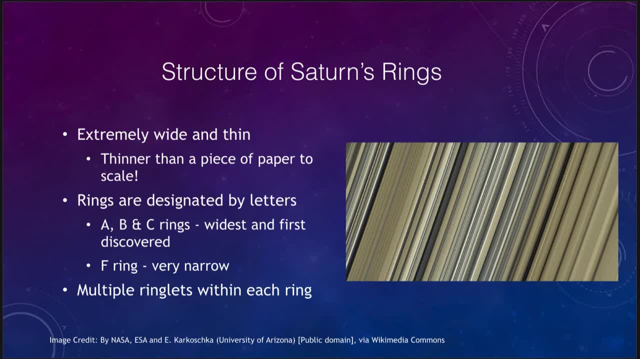 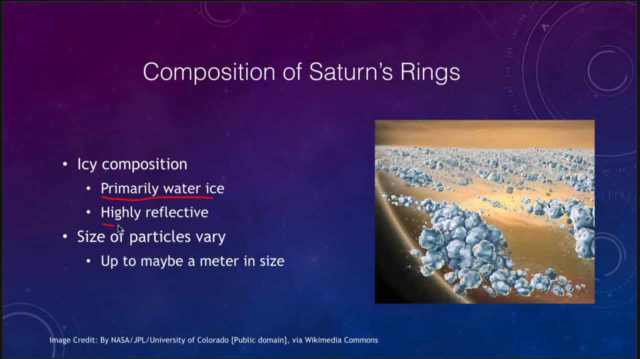 We'll come back and look at that shortly. So let's look here at the compositions. What are these made up of? Saturn's rings are primarily water, ice, which makes them highly reflective. So why do we see them prominently from Earth? Because they're reflecting a lot of light. 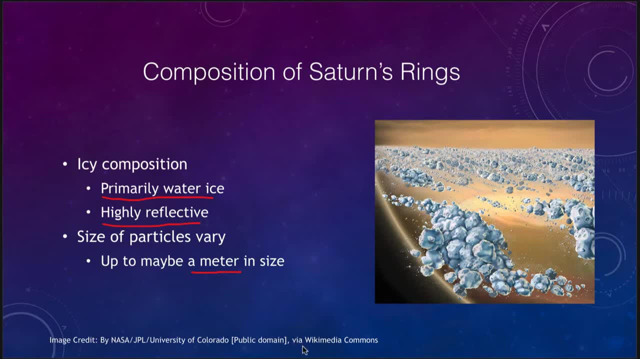 The size of the Part Particles Varies: may be up to about a meter in size, and some of them will clump together. Now, this is an artist's conception of what the rings might look like if you were sitting there. 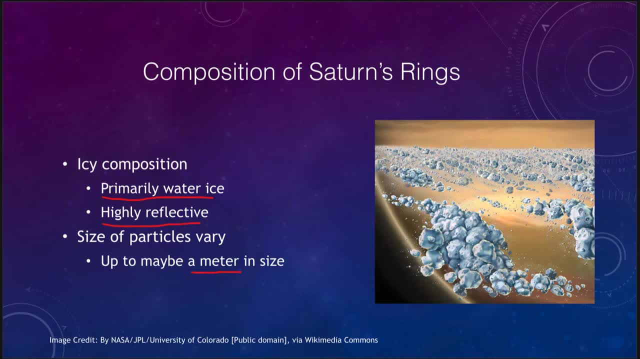 inside the rings of Saturn themselves. So you'd have clumps of material and these would likely stick together. They're not strong enough to really hold themselves together gravitationally, So as objects collide they would stick together and other times they would be pushed apart. 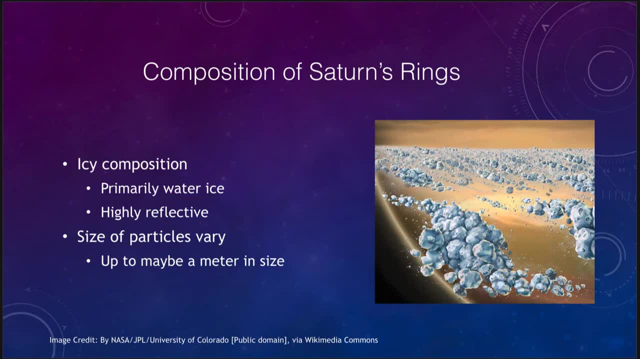 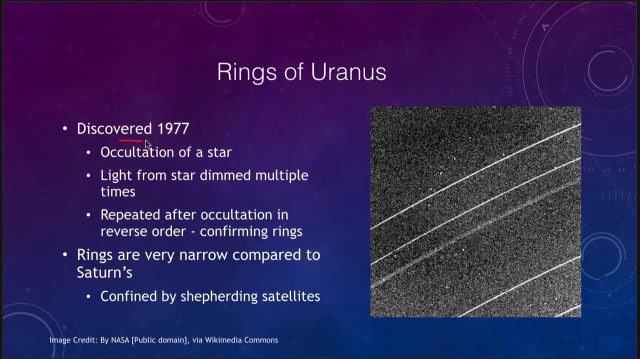 Saturn again has the primary and most detailed rings, but the other objects have rings as well. So let's look at Uranus here. Uranus's rings were discovered in 1977, a couple of years before Jupiter's were discovered. 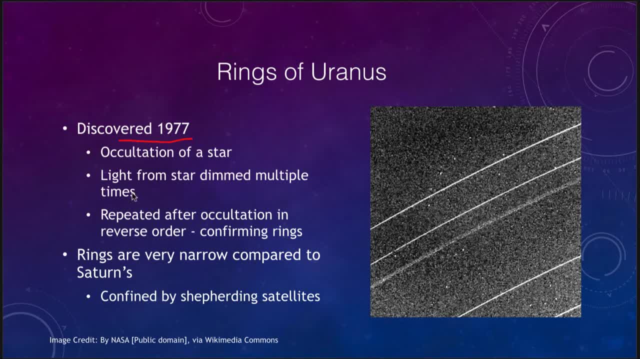 although hundreds of years after the rings of Saturn were known, They were discovered during the occultation of a star. What happened was Uranus was going to pass in front of a star, so astronomers wanted to study how its light dimmed as well. 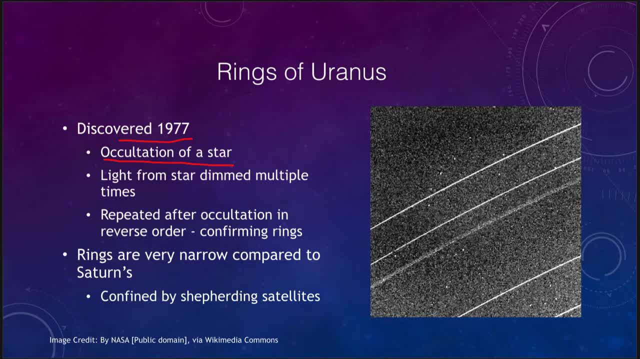 as it passed in front of, as the star, as it passed in front of the star, But before the planet passed in front of the star, we saw that the light dimmed multiple times And this repeated after the occultation, in the reverse order, kind of confirming. 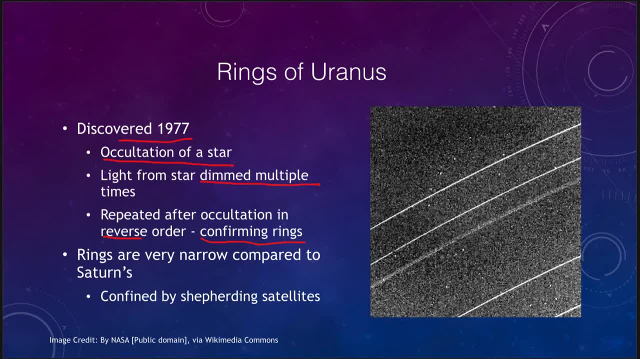 that the rings did. the rings did exist, So the rings, as the star was passing, the rings would pass in front of the star and that would dim the light a little bit as each of these rings passed in front of the star. 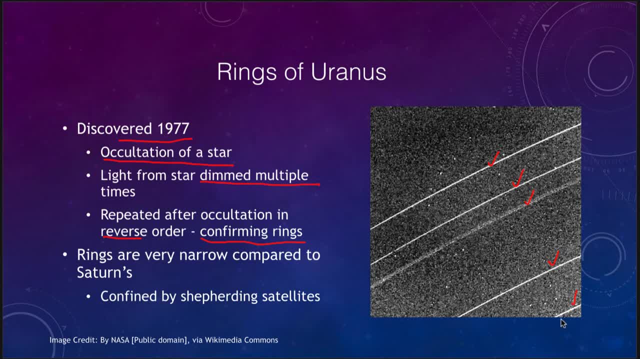 in turn, And then you can imagine on the other side. you went the other direction and it would pass through the rings in the opposite order. Rings are extremely narrow compared to the rings of Saturn, So we see the rings of Uranus here very, very thin. 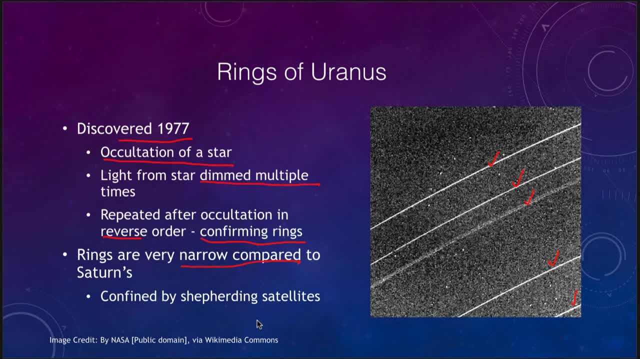 These are not the wide, broad rings that we saw of Saturn. They are actually confined by shepherding satellites, little moons that will orbit just on one side and just on the other side and keep all those particles in line, So essentially, as one moon orbits and the other moon. 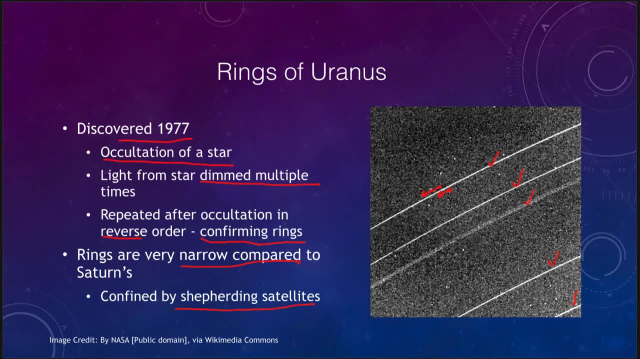 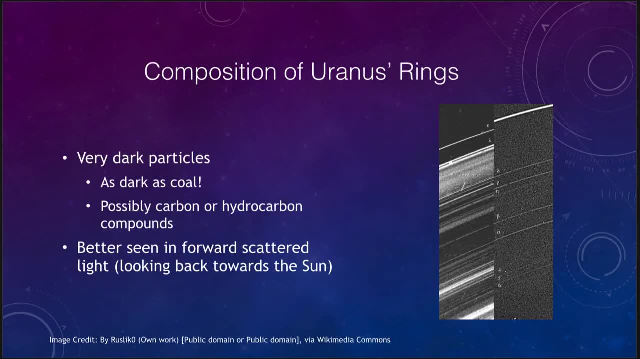 orbits. their gravity will keep those very well confined. Now, what is the composition of these rings? Well, they are very dark particles. Again, why do we not see them from Earth? They're not icy like the rings of Saturn. They are in fact as dark as coal. 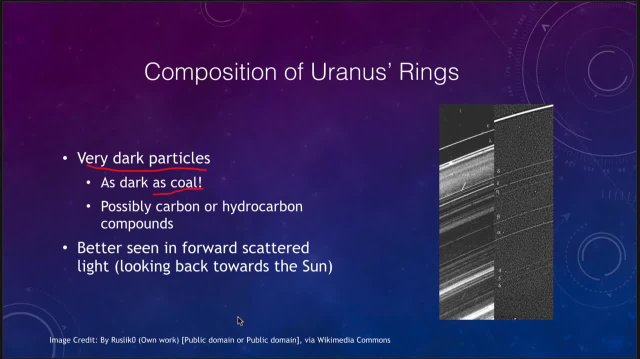 So we don't really see them in forward. in looking forward, We do see them in forward- scattered light, which means we're looking back towards the sun. So if we look at the image here, there is what we see of the rings from the Earth. 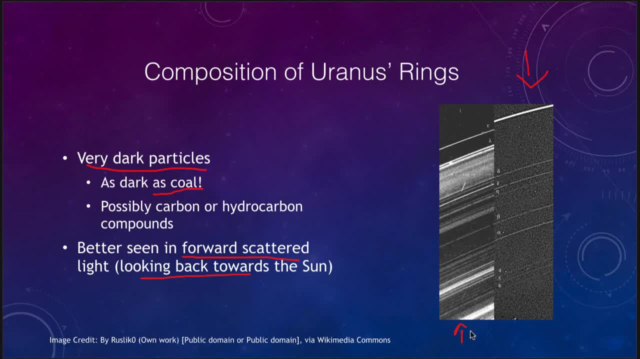 But if we were behind them, looking back, we would see all sorts of light scattering through these rings. So there are a lot more structures there that we don't actually see from Earth, but that we had to get around behind, And the only object that really went close. 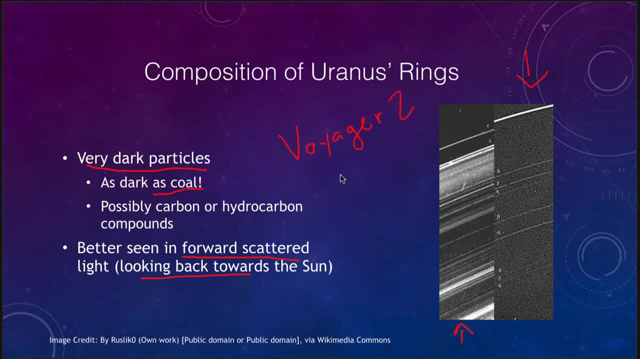 to this was the Voyager 2 spacecraft that actually went past Uranus and was able to turn back and look back to the sun. But it's a very different structure you get if you're looking from the sun versus if you're looking from behind. 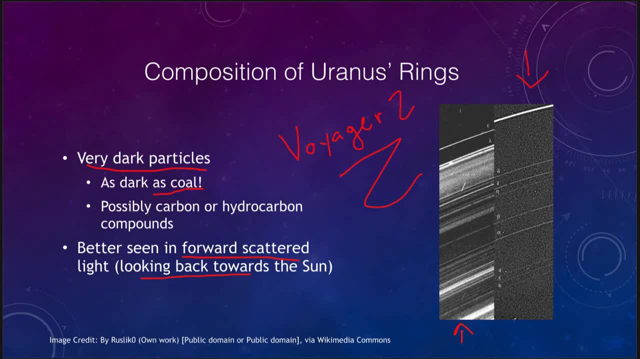 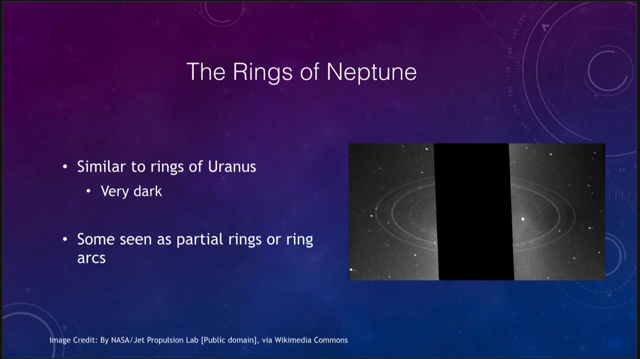 When you look from behind, other than the composition we know is different, we see very similar structures to what we saw on Saturn. Now, the last of the objects to look at with rings would be Neptune. Neptune has very, very dark rings. 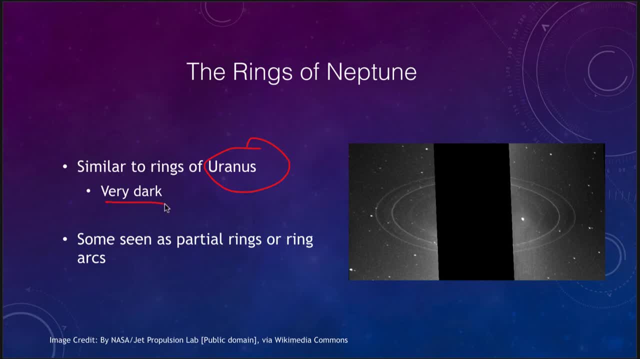 in many ways similar to those of Uranus, and they are quite dark And we can see them here. This is blocking out the light from the planet, which would overwhelm the very faint rings. So they're there, but we've got to block out the planet's light. 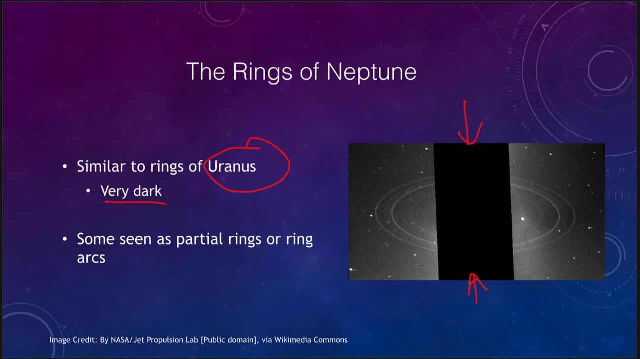 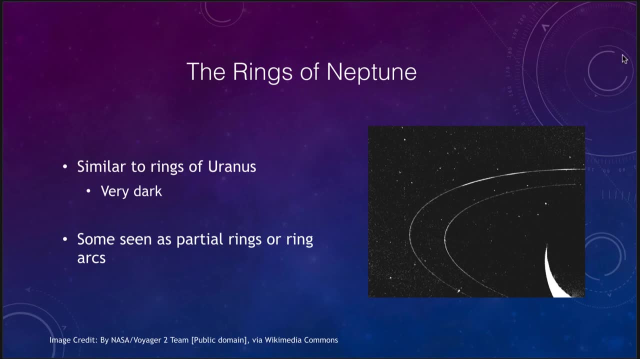 in order to even be able to see them. They are seen as arcs sometimes. So if we look here another image of it and we see that there are denser areas of the rings and there are areas where there is less ring material, 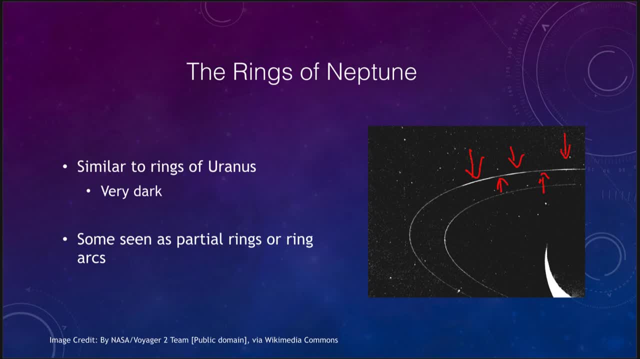 So, unlike the rings of Saturn and Uranus, which seem to be relatively smooth, the rings of Neptune are sometimes seen as partial rings or even just ring arcs. So there's a little bit of a difference there in Neptune. Are these relatively young or relatively old rings? 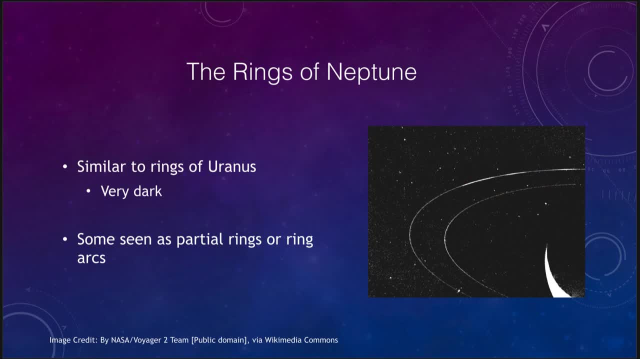 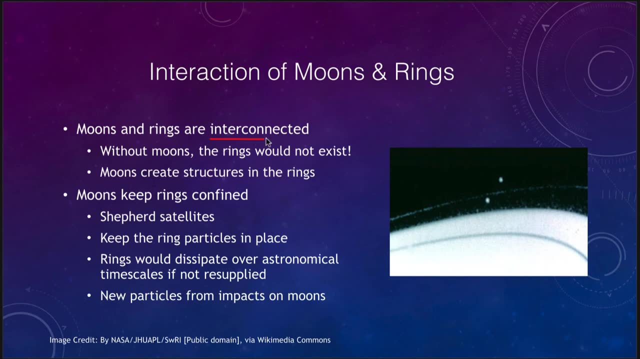 Something we really do not know. Now, the last thing We want to look at is the interactions between the moons and the rings. There is an interconnection between these And, in fact, without the moons, the rings would not exist. Where did the rings come from? 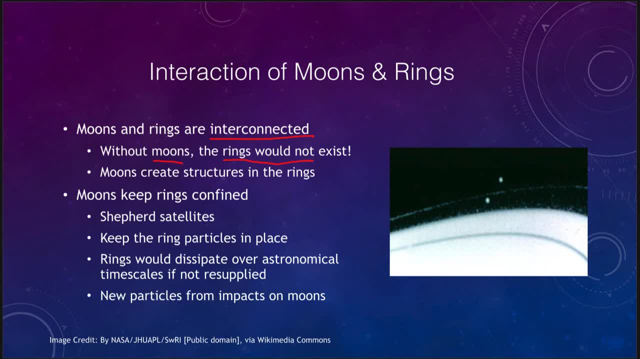 Probably from particles blasted off the moons in impacts, And that would then give the rings particles, a supply of material. The moons also keep the rings confined and that's what we call the shepherding satellites Which we see here orbiting around and keeping. 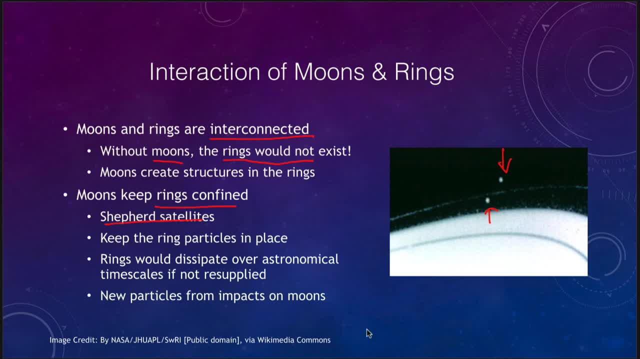 this: the ring particles in this very narrow ring, well confined, So they keep the ring particles in place. The rings would dissipate over astronomical time scales. If we run models of all these particles orbiting, we would find that they would slowly dissipate out into space. 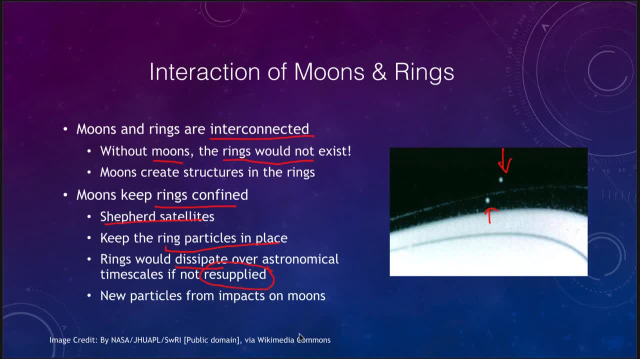 There has to be some form of resupply, and that would be from the moons. That impacts On the moons could actually throw more material back into them and replenish the ring particles. So where do we get those new particles from impacts on the moons?